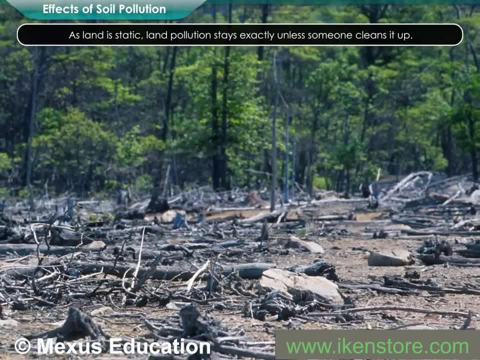 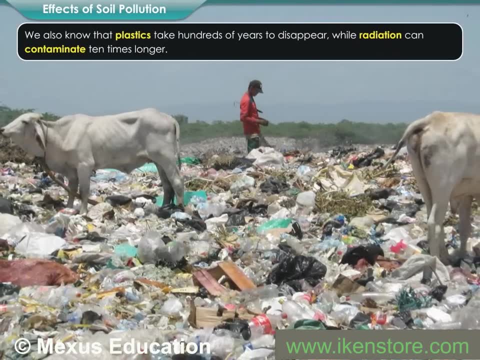 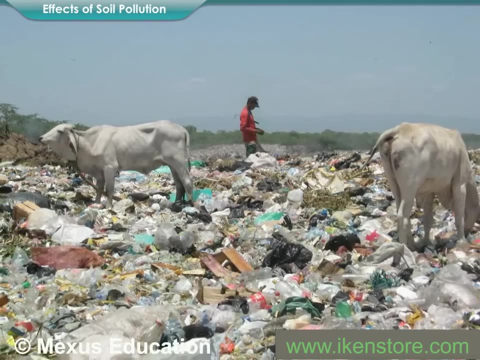 As land is static, land pollution stays exactly unless someone cleans it up. We also know that plastics take hundreds of years to disappear, While radiation can contaminate ten times longer. The simplest effect of land pollution is that it takes land out of circulation. 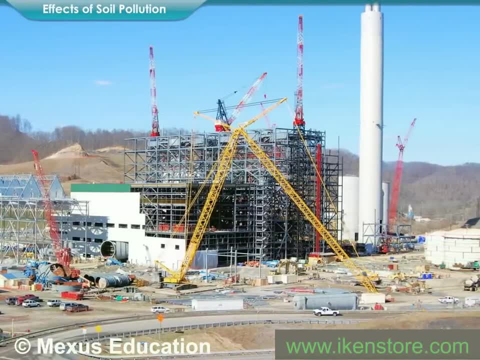 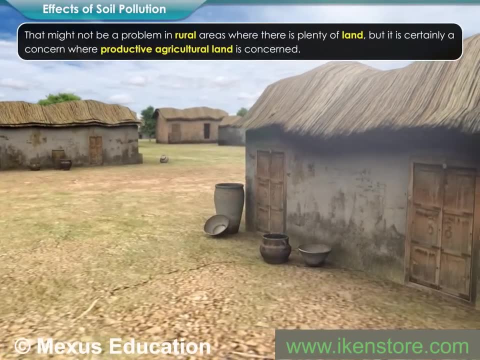 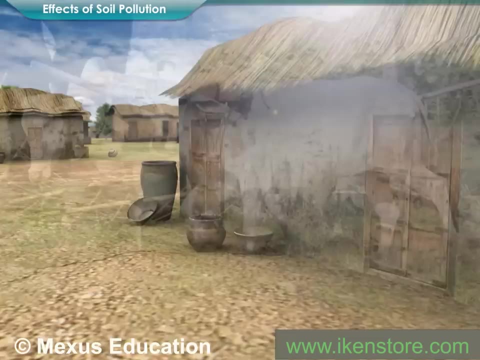 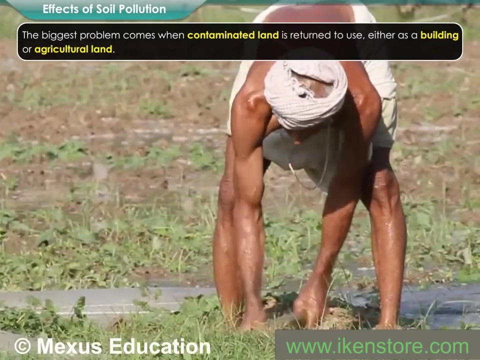 That is, the more land we use up, the less we have remaining. That might not be a problem in rural areas where there is plenty of land, But it is certainly a concern where productive agricultural land is concerned. The biggest problem comes when contaminated land is returned to use either as a building or agricultural land. 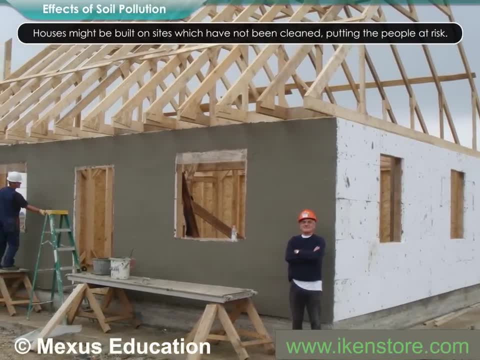 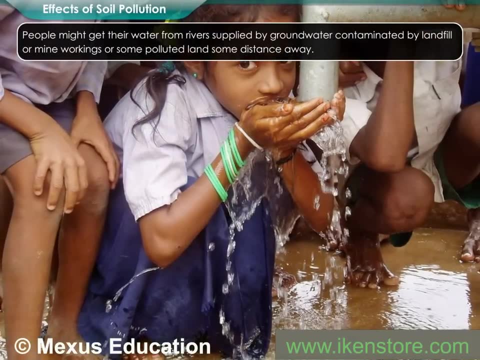 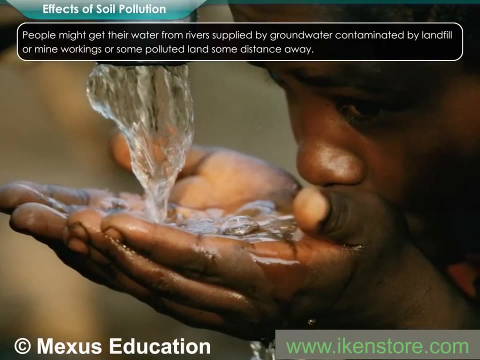 Houses might be built on sites which have not been cleaned, putting the people at risk. People might get their water from rivers supplied by groundwater contaminated by landfill or mine workings or some polluted land And, as a result, they find themselves having to claim the land for their land. 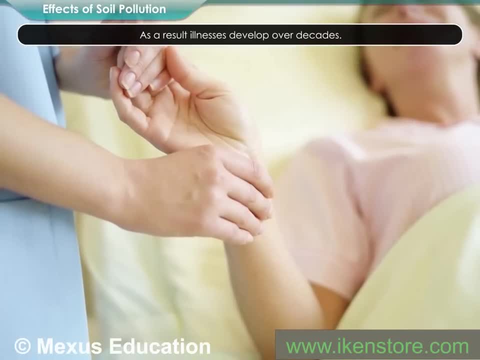 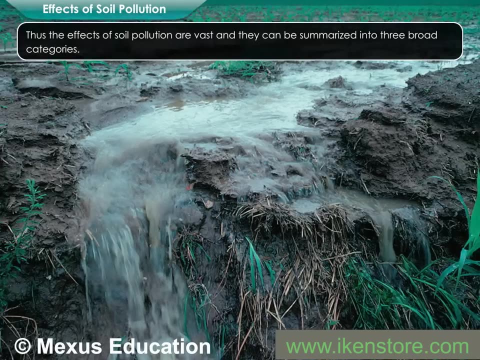 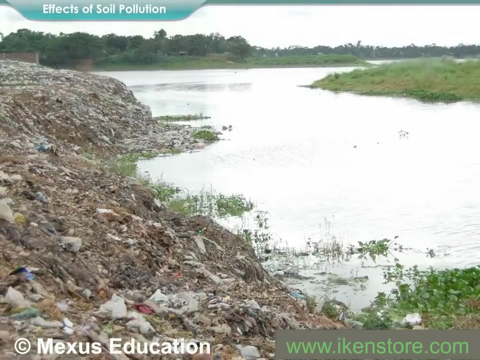 The only way to solve this is to put their homes and houses under protection. The ones that do not even have a project are provided with land that are not protected from air pollution, as well as any other chemical or chemical agents. These precisamente cause soil pollution to be so severe that there are some native plants and plants to be protected from it. 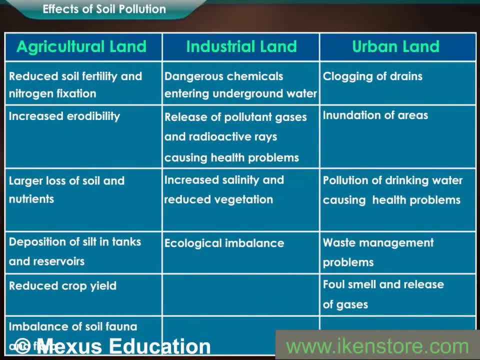 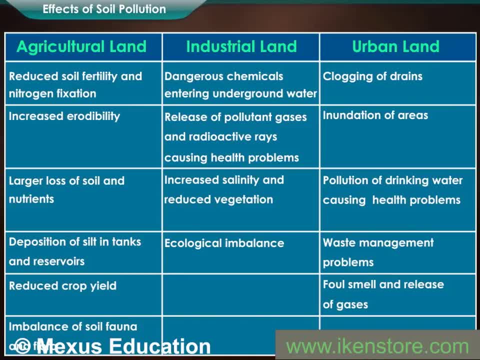 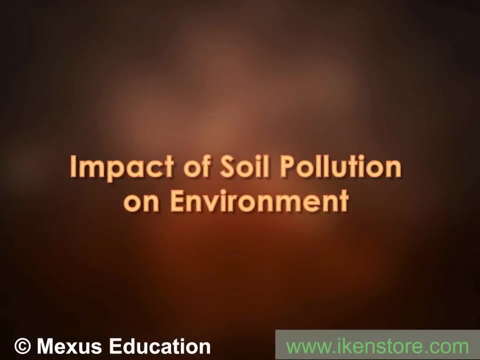 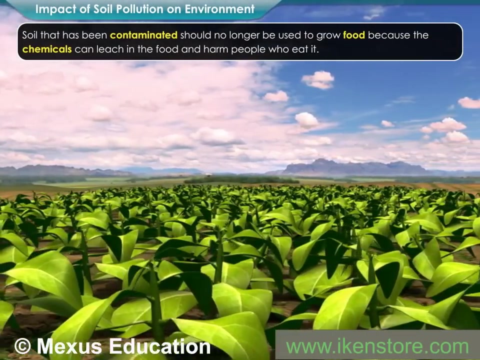 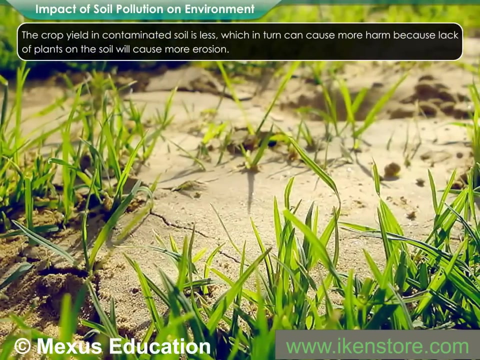 Soil that has been contaminated should no longer be used to grow food, because the chemicals can leach in the food and harm people who eat it. The crop yield in contaminated soil is less, which in turn can cause more harm because lack of plants on the soil. 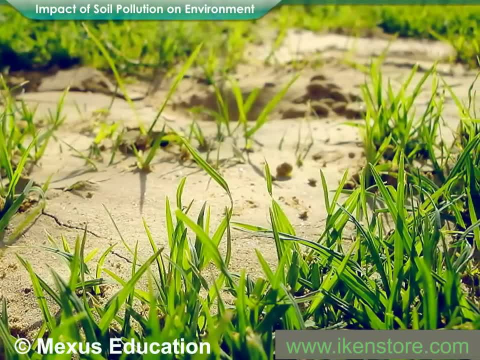 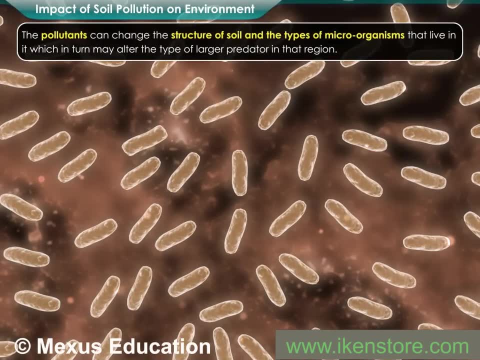 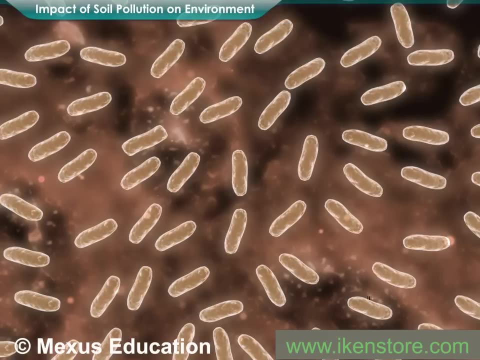 will cause more erosion. In addition, the pollutants can change the structure of soil and the types of microorganisms that live in it, which in turn may alter the type of larger predator in that region. Thus, soil pollution can change the whole ecosystem. 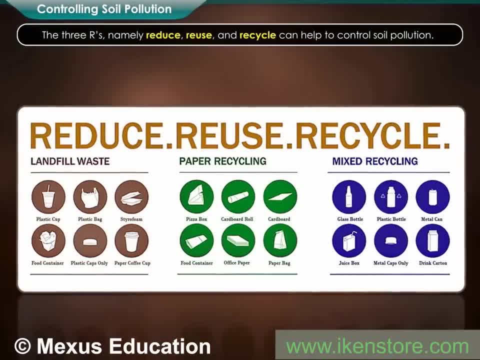 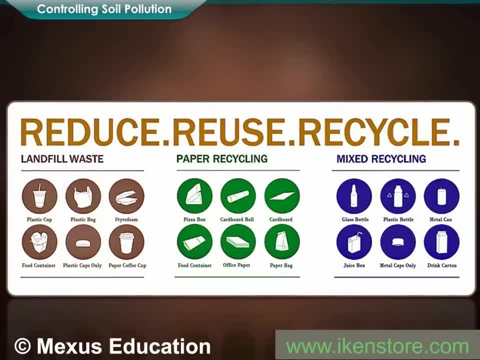 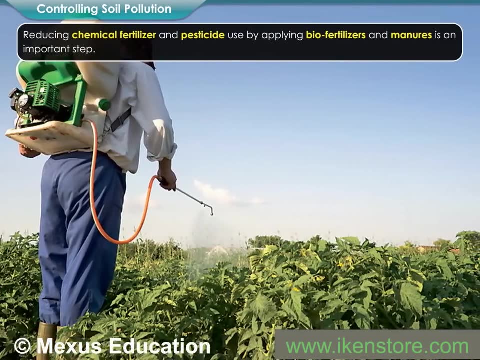 The three R's, namely reduce, reuse and recycle, can help to control soil pollution. Reducing the use of soil pollution and the use of chemical fertilizer and pesticide by applying biofertilizers and manures is an important step to control soil pollution. 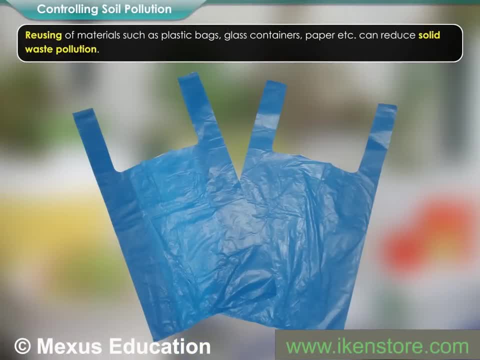 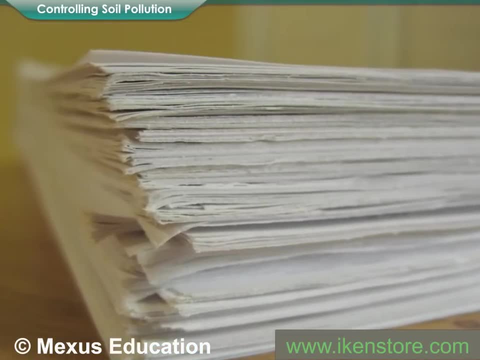 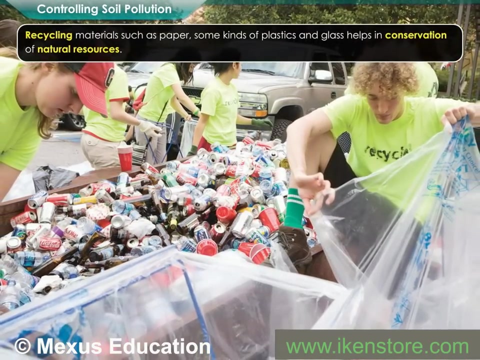 Reusing of materials such as plastic bags, glass containers, paper, etc. can reduce solid waste pollution. Recycling materials such as paper, some kinds of plastics and glass helps in conservation of natural resources. Recycling materials such as plastic bags, some kinds of plastics and glass. 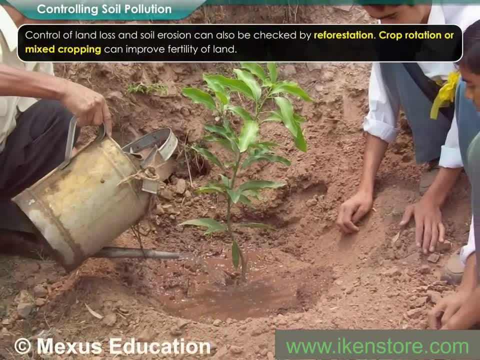 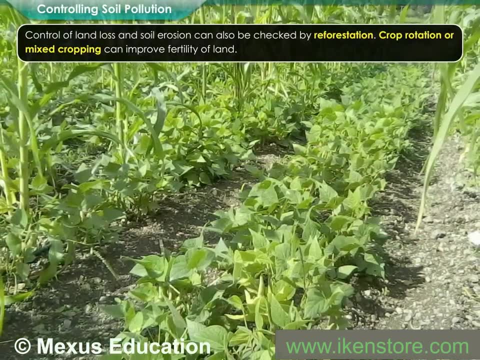 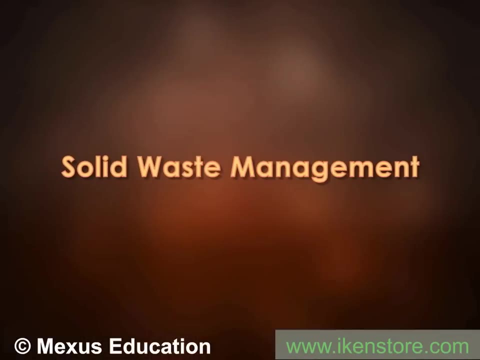 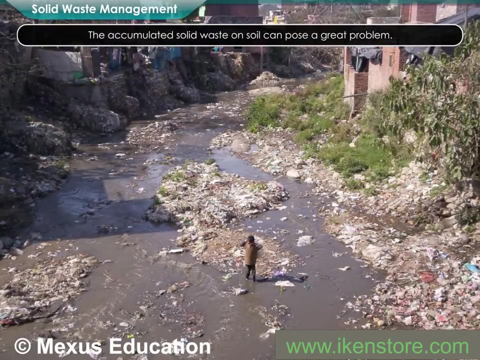 helps in conservation of natural resources. Control of land loss and soil erosion can also be checked by reforestation. crop rotation or mixed cropping can improve fertility of land can improve fertility of land. The accumulated solid waste on soil can pose a great problem. 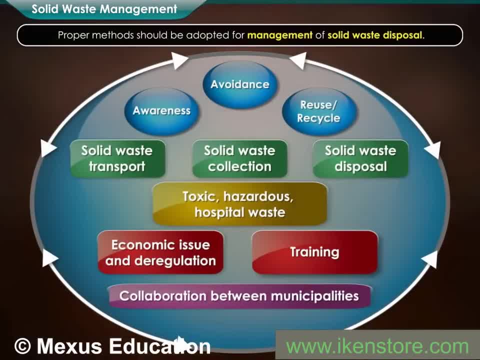 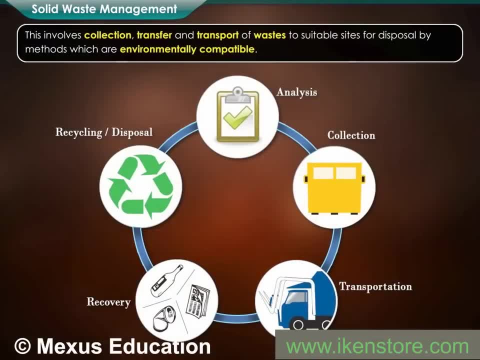 Hence soil pollution can be reduced. Hence proper methods should be adopted for management of solid waste disposal. for management of solid waste disposal, This involves collection, transfer and transport of wastes. This involves collection, transfer and transport of wastes to suitable sites for disposal by methods. 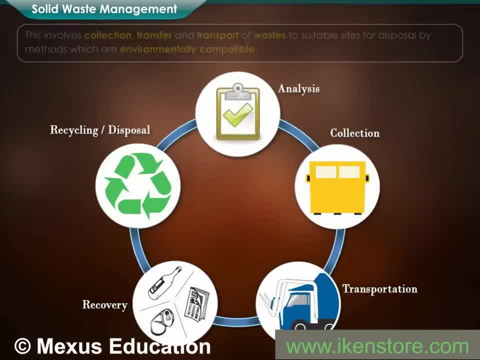 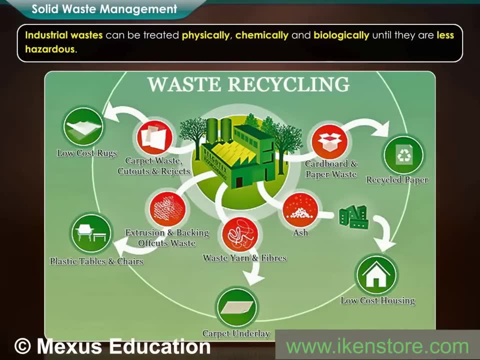 which are environmentally compatible, which are environmentally compatible. Industrial waste can be treated physically, chemically and biologically until they are less hazardous. until they are less hazardous. Until they are less hazardous, Acidic and alkaline waste can be used as a source of waste. 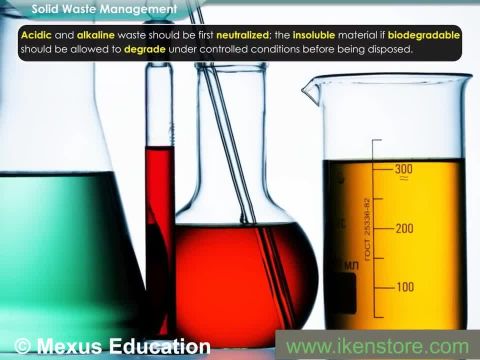 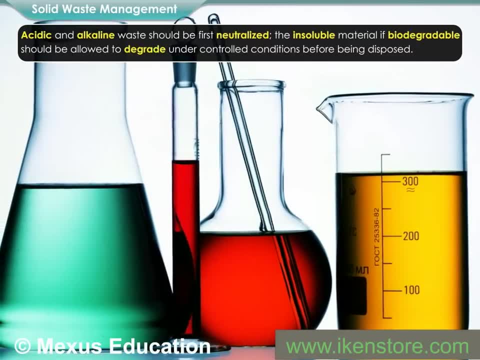 Acidic and alkaline waste can be used as a source of waste. Alkaline waste should be first neutralized. The insoluble material, if biodegradable, should be allowed to degrade under controlled conditions before being disposed. New areas for storage of hazardous waste. 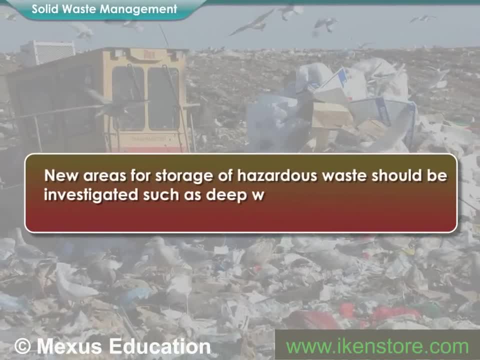 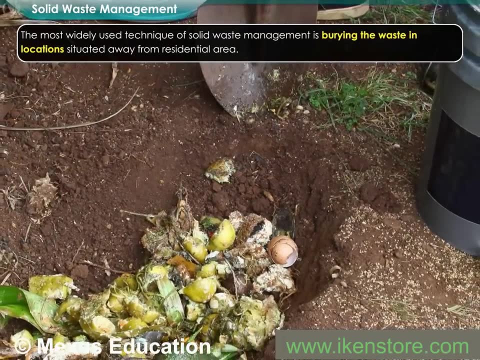 New areas for storage of hazardous waste should be investigated, such as deep well injections and more secure landfills. and more secure landfills: The most widely used technique of solid waste management. The most widely used technique of solid waste management is barring the waste in locations situated. 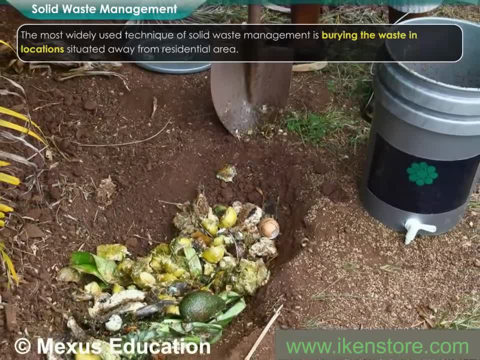 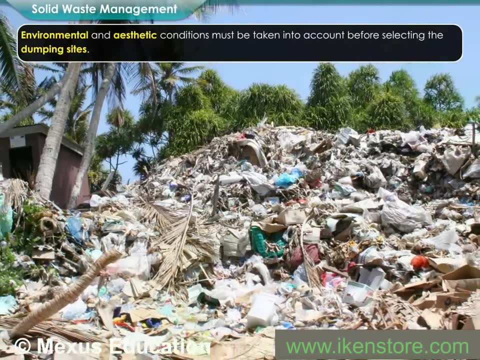 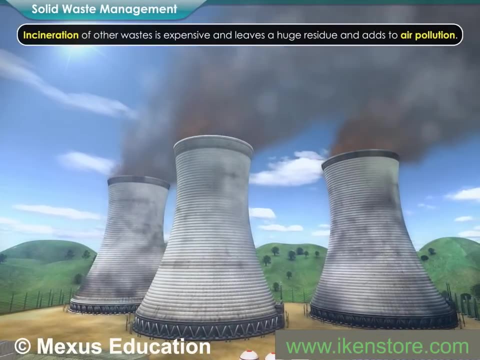 is barring the waste in locations situated away from residential area, away from residential area. Environmental and aesthetic conditions must be taken into account before selecting the dumping sites. before selecting the dumping sites, Incineration of other wastes is expensive and leaves a huge residue. 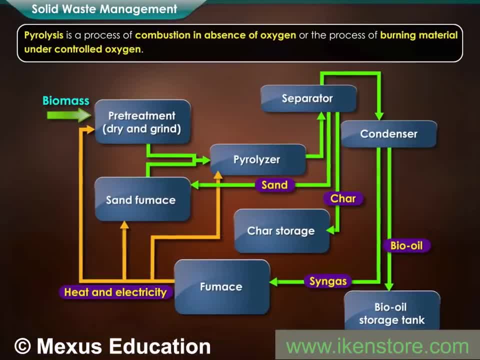 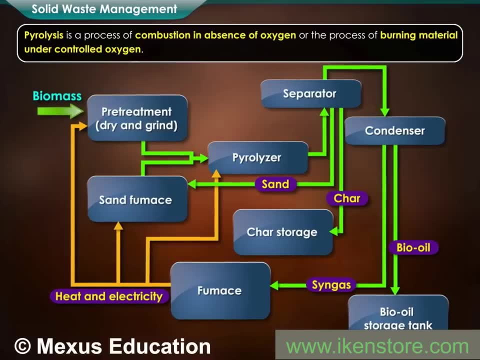 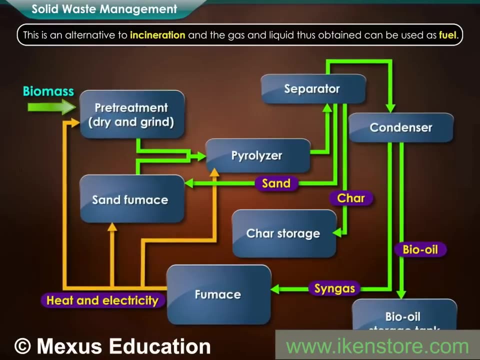 and adds to air pollution. Pyrolysis is a process of combustion and adds to air pollution. Pyrolysis is a process of combustion in the process of burning material under controlled oxygen. This is an alternative to incineration, and the gas and liquid thus obtained. 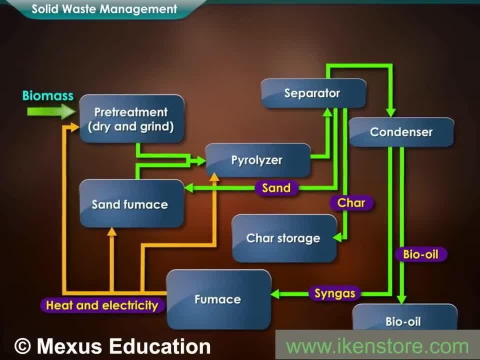 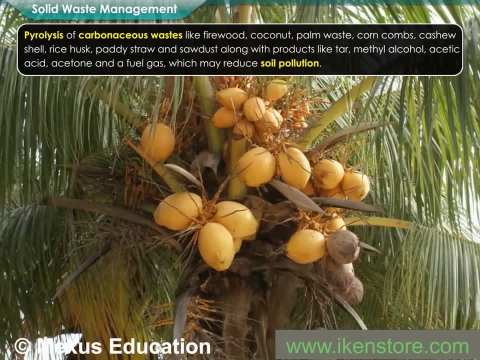 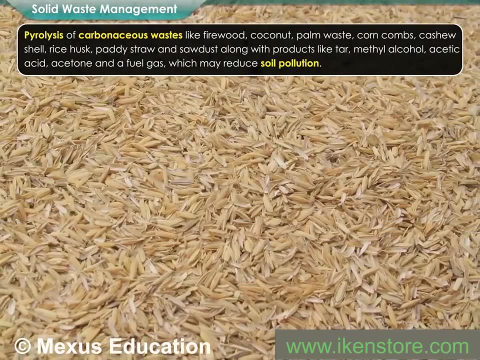 and the gas and liquid thus obtained can be used as fuel. Pyrolysis of carbonaceous wastes. Pyrolysis of carbonaceous wastes like firewood, coconut, palm waste, corn combs, cashew, shell, rice, husk, paddy straw. 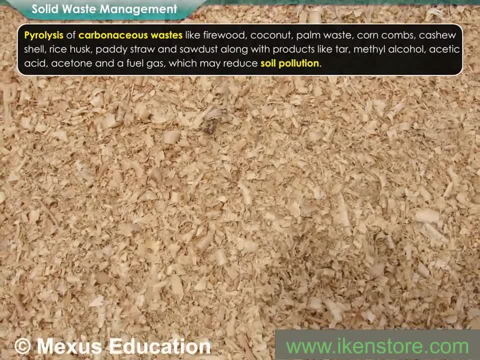 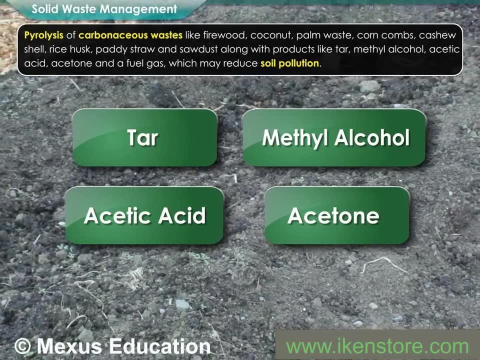 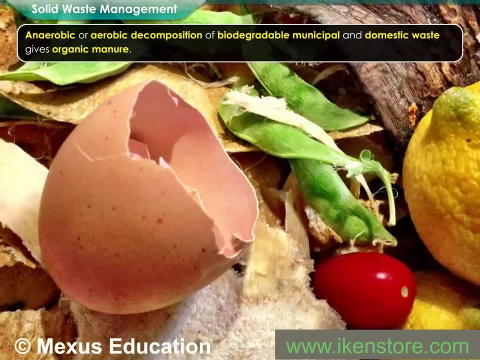 and sawdust yields charcoal, along with products like tar, methyl alcohol, acetic acid, acetone and a fuel gas which may reduce soil pollution, which may reduce soil pollution. Anaerobic or aerobic decomposition of biodegradable municipal and. 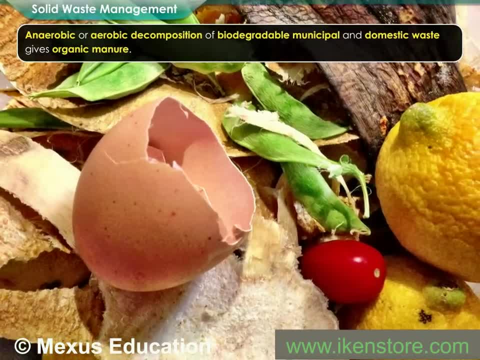 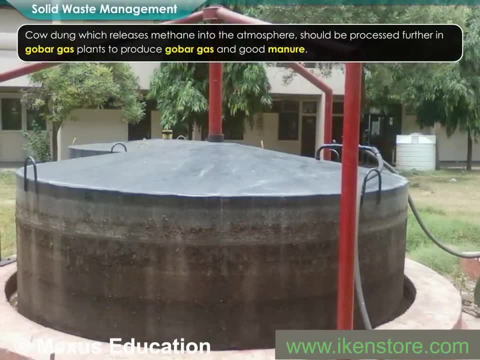 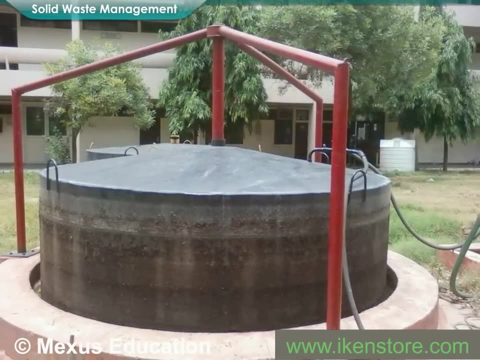 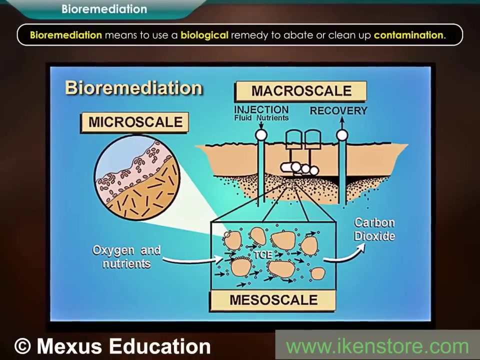 domestic waste gives organic manure. Cow dung, which releases methane into the atmosphere, should be processed further in gober gas plants to produce gober gas and good manure. Bioremediation means to use a biological remedy to abate or clean up contamination. 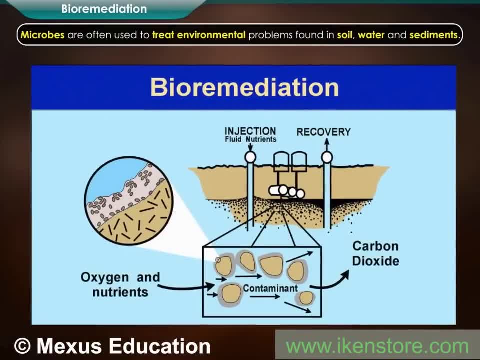 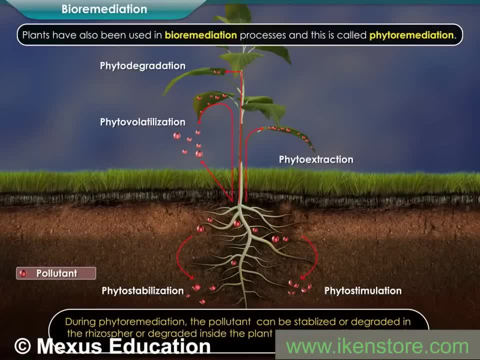 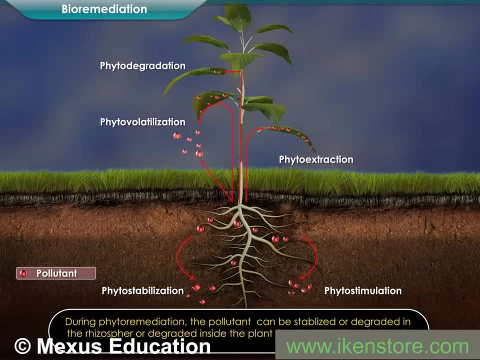 Microbes are often used to treat environmental problems found in soil, water and sediments. Plants have also been used in bioremediation processes, and this is called phytoremediation. Biological processes have been used for some inorganic materials like metals. 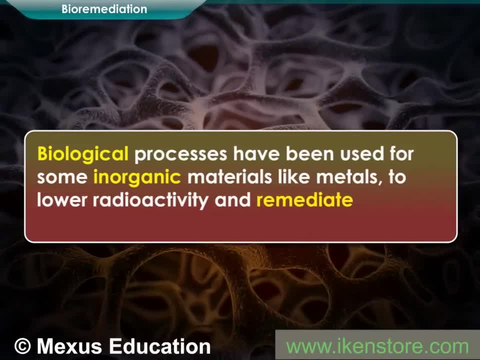 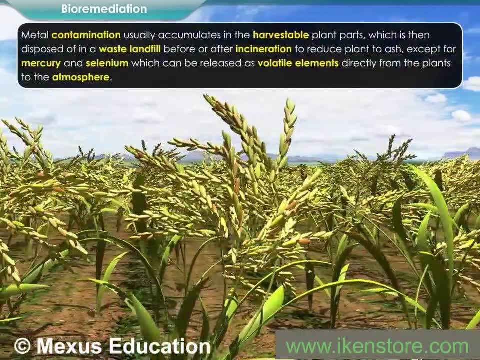 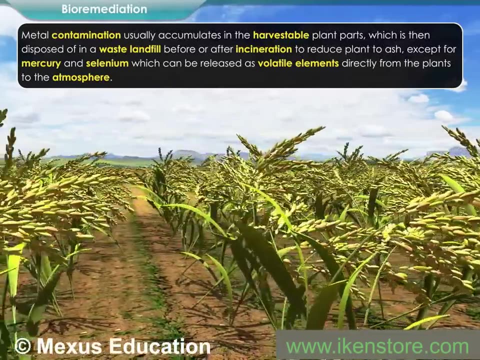 to lower radioactivity and remediate inorganic contaminants. Metal contamination usually accumulates in the harvestable plant parts, which is then disposed off in a waste landfill before or after incineration to reduce the plant to ash, Except for mercury and selenium, which can be released, 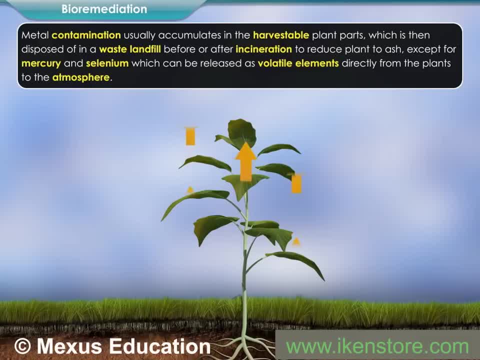 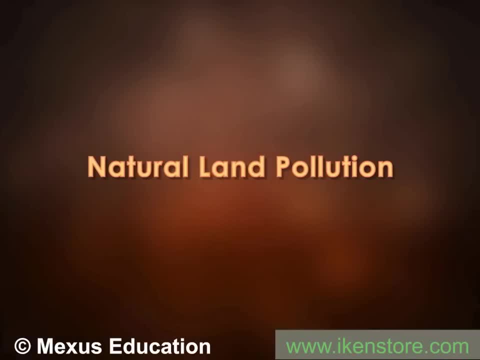 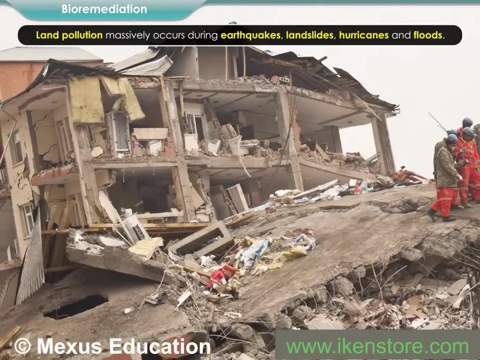 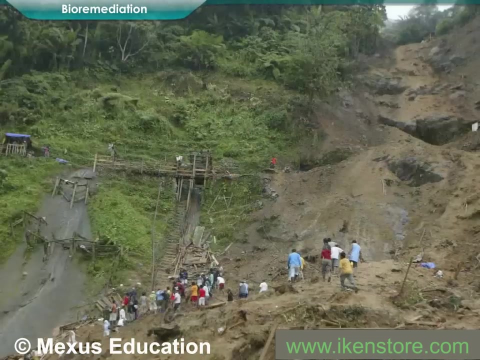 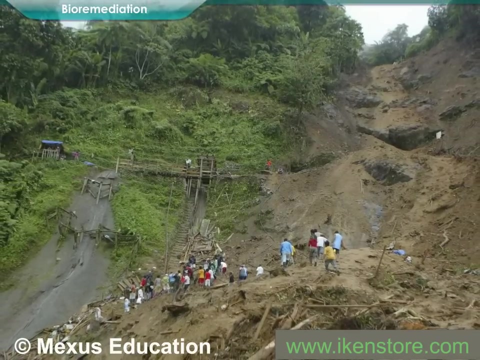 as volatile elements directly from the plants to the atmosphere. Land pollution massively occurs during earthquakes, landslides, hurricanes, floods. Cleaning of land in such situations becomes difficult and expensive. Also, it may take years to restore the affected area. These kinds of 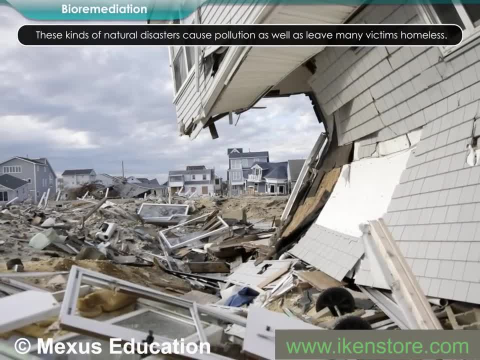 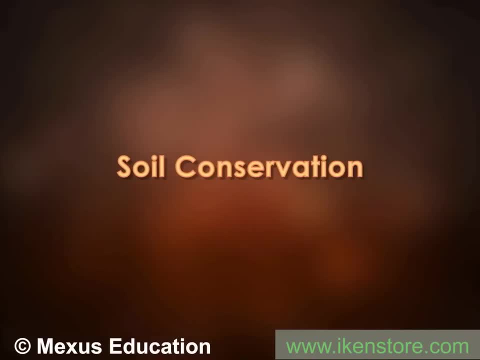 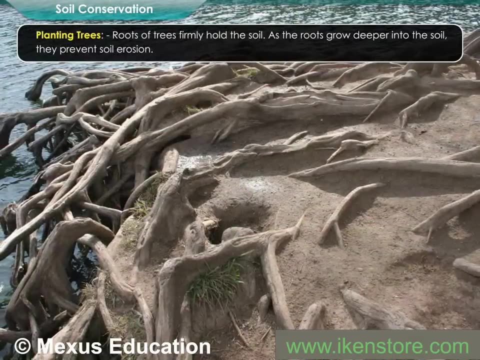 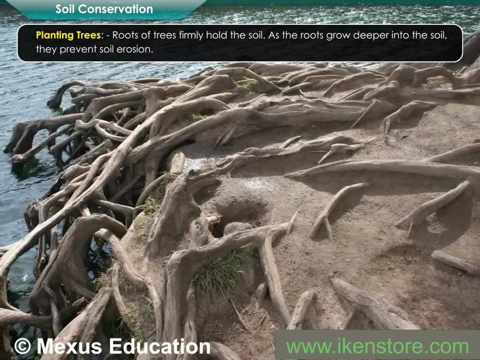 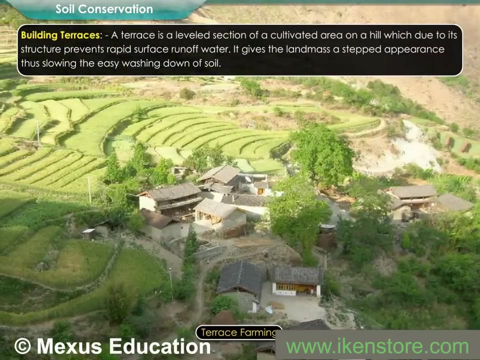 of natural disasters cause pollution as well as leave many victims homeless. there are several ways of soil conservation: planting trees: roots of trees firmly hold the soil. as the roots grow deeper into the soil, they prevent soil erosion. building terraces: a terrace is a leveled section of a cultivated area. 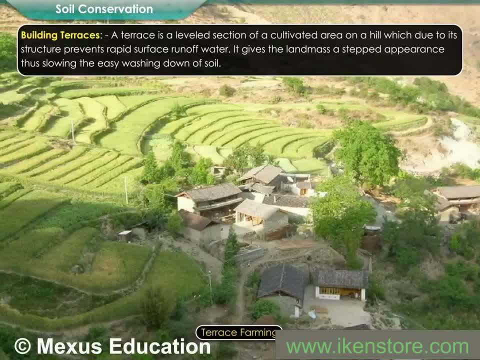 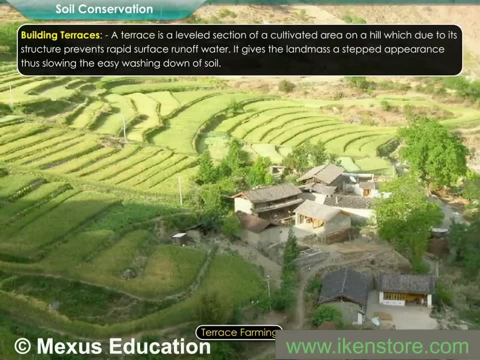 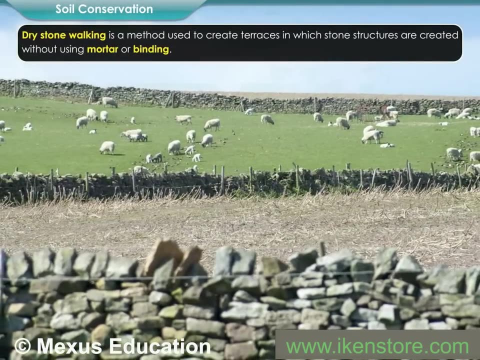 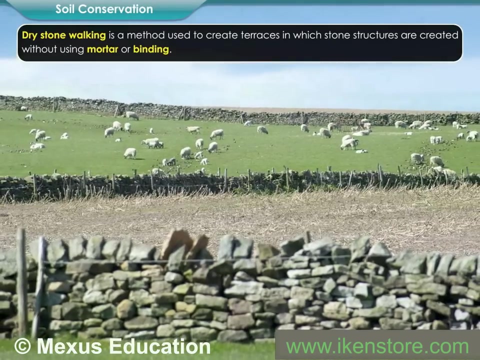 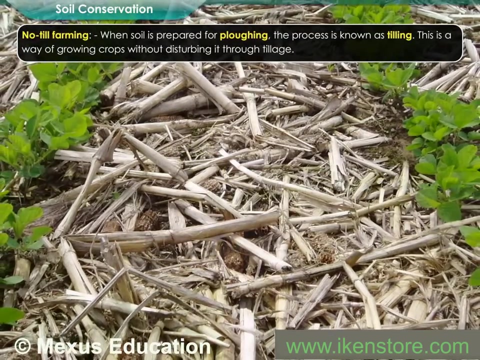 on a hill which, due to its structure, prevents a rapid surface runoff water. it gives the landmass a stepped appearance, thus slowing the easy washing down of soil. dry stone walking is a method used to create terraces in which stone structures are created without using mortar or binding. no till farming. when soil is prepared for plowing, the process is: 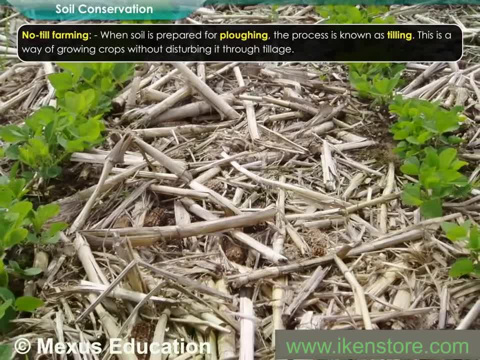 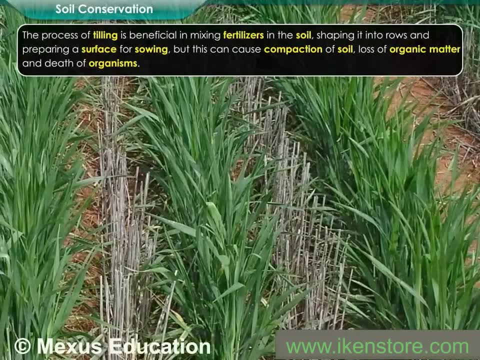 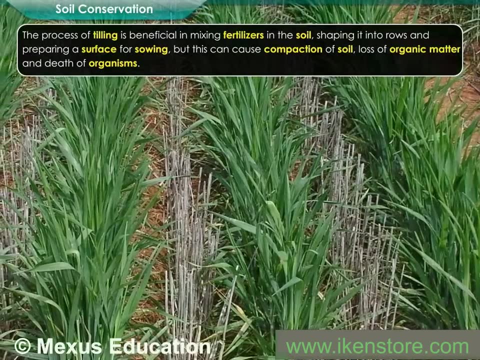 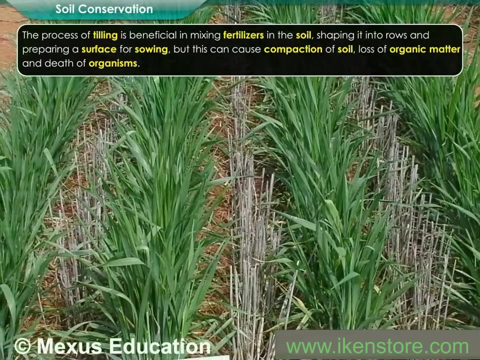 known as tiling. this is a way of growing crops without disturbing it through tile it. the process of tiling is beneficial in mixing fertilizers in the soil, shaping it into rows and preparing a surface for sewing, but this can cause compactions of soil, loss of organic matter and death of organisms. contour plowing this practice.